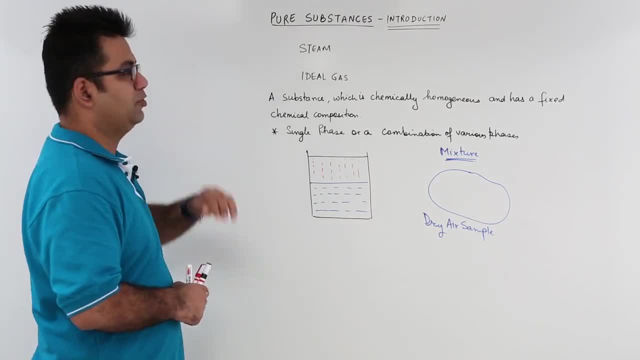 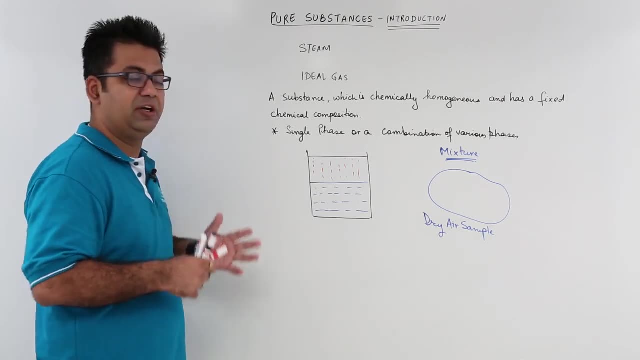 Now in this video we will start understanding that. what is a pure substance? So we will introduce the term pure substance in this video. There are two very important working fluids that we deal with in thermodynamics, So the first one is steam and the other one is an ideal. 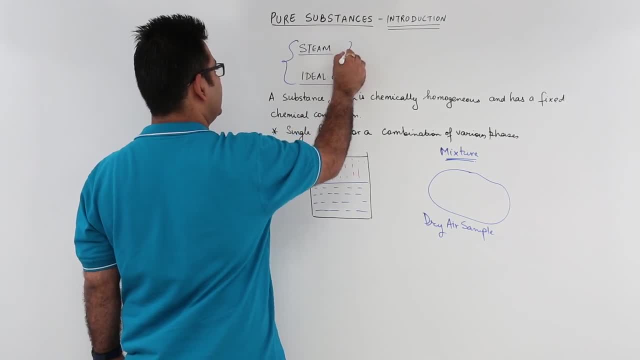 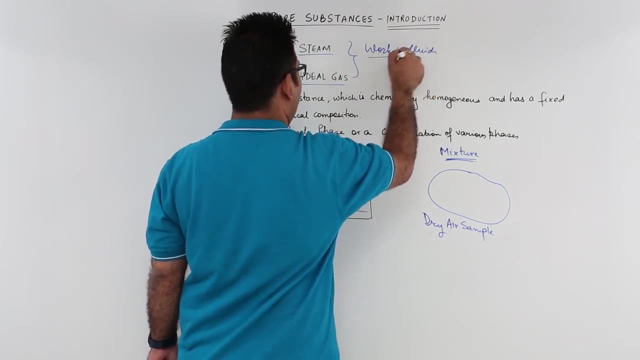 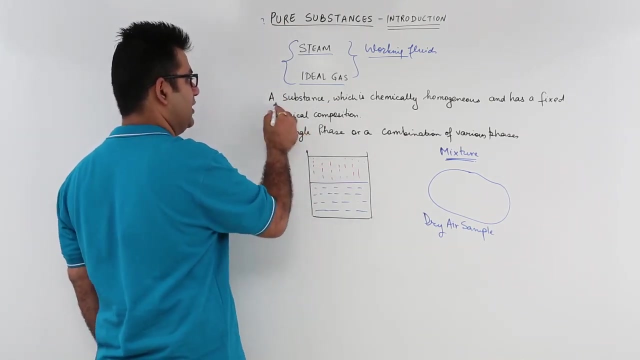 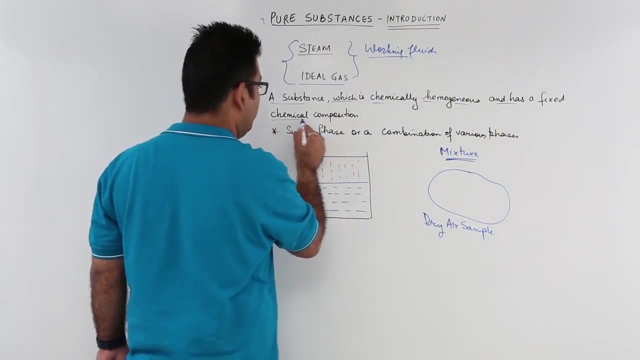 gas. So these are two things which we term as the working fluids, And to understand their properties, you must understand that what is a pure substance? To define it, a pure substance is a substance which is chemically homogeneous and has a fixed chemical composition throughout. 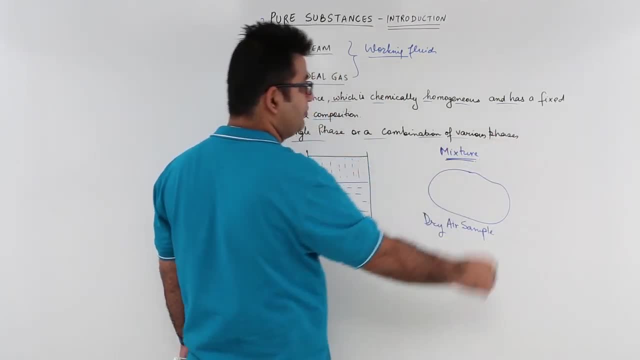 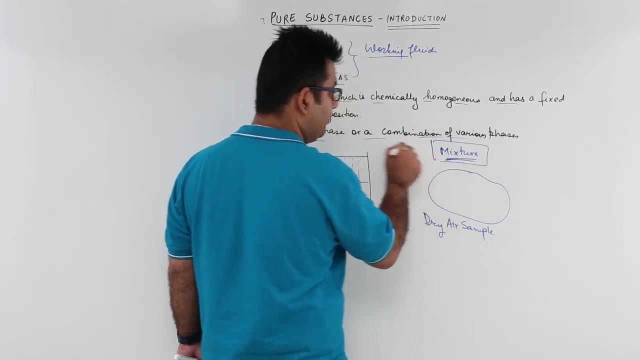 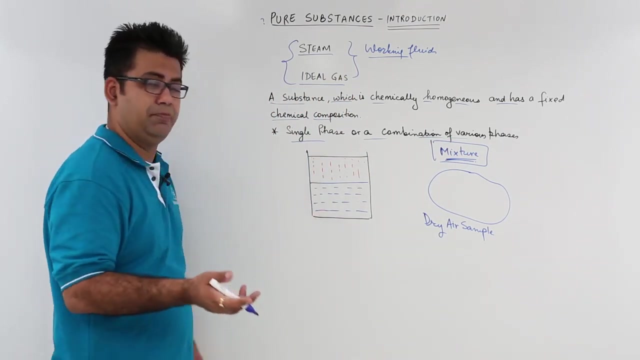 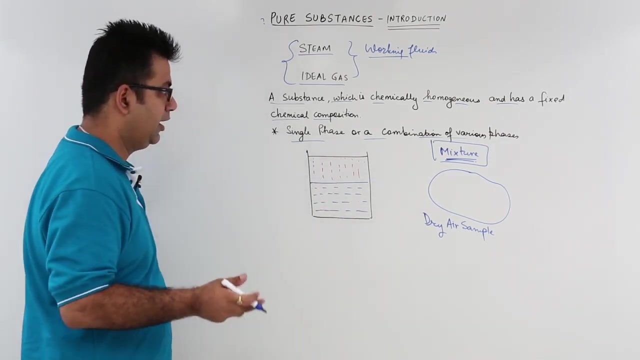 It might be present in a single phase or in a combination of various phases, And a pure substance can also be a mixture. So we talk about how you know a single phase, which is you know, but obviously understood, how a combination of various phases becomes a pure substance. For example, if I have only 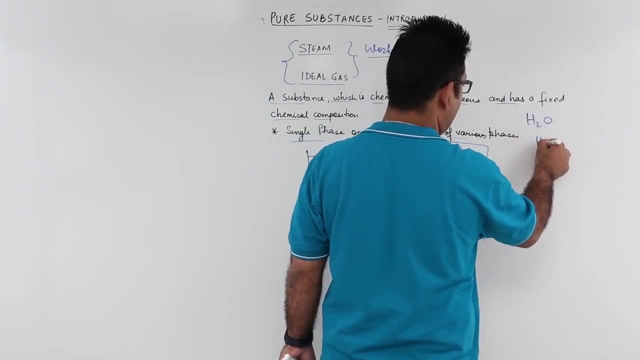 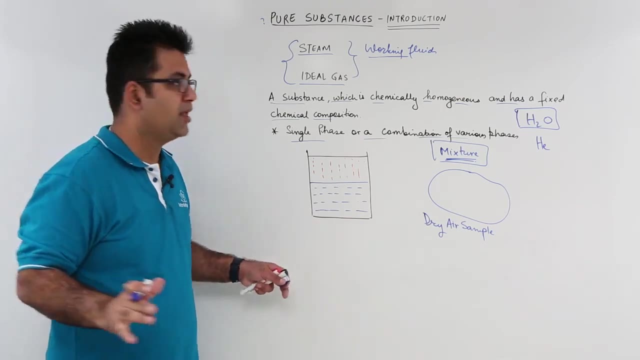 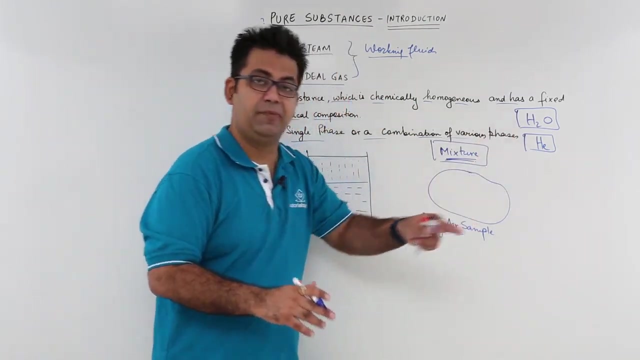 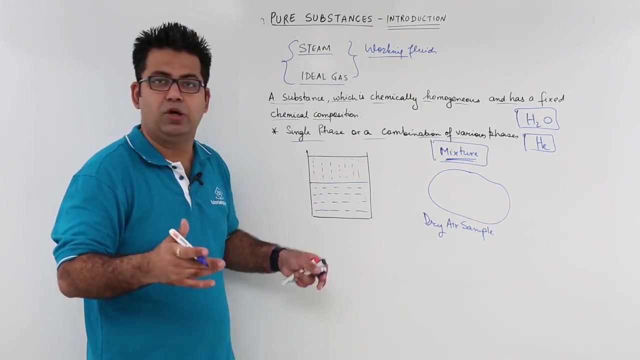 water, if I have only water or if I have only helium. So water will have constant chemical composition throughout and helium also will be chemically you can say, homogeneous throughout. So these two substances can be termed as a pure substance. Now, if you have, you can say liquid water, then 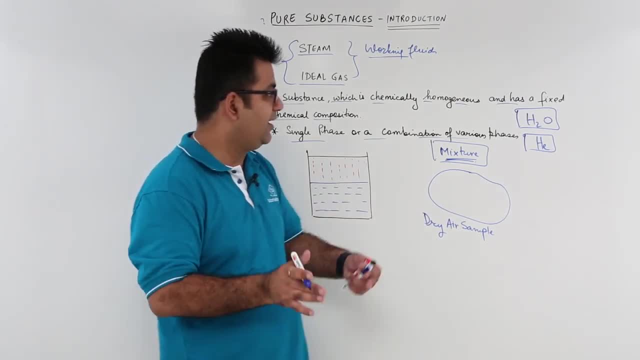 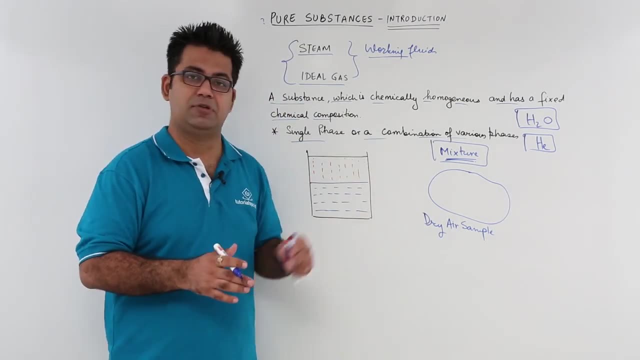 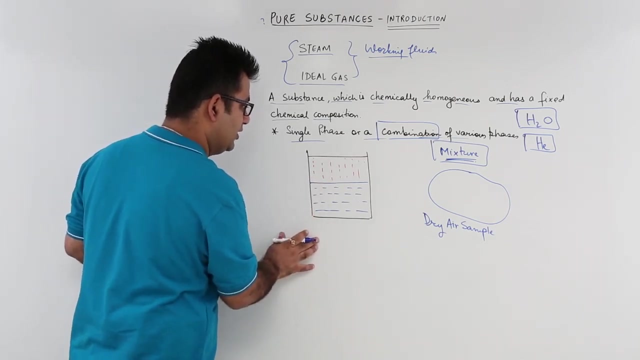 yes, it's a single phase, entirely pure substance. If you have liquefied helium, also entirely single composition throughout and is termed as a pure substance. But what about if you have a combination of various phases? Okay, let's have a look at that in this figure over. 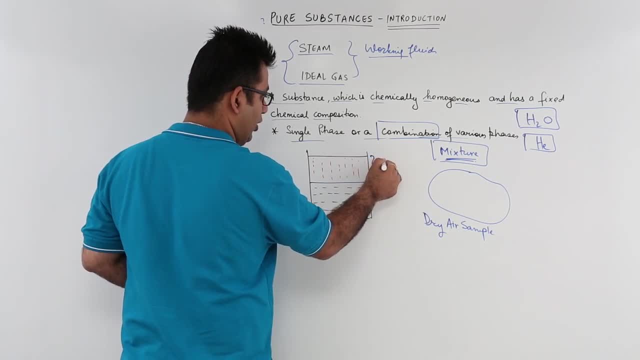 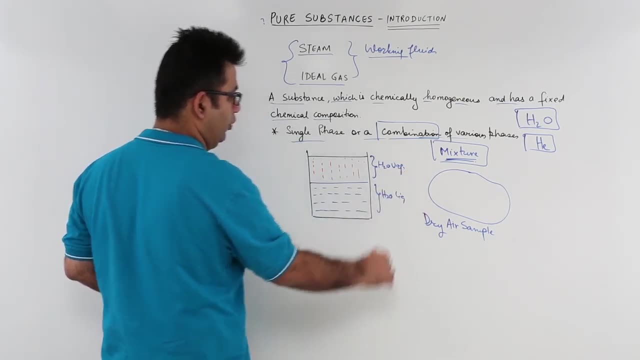 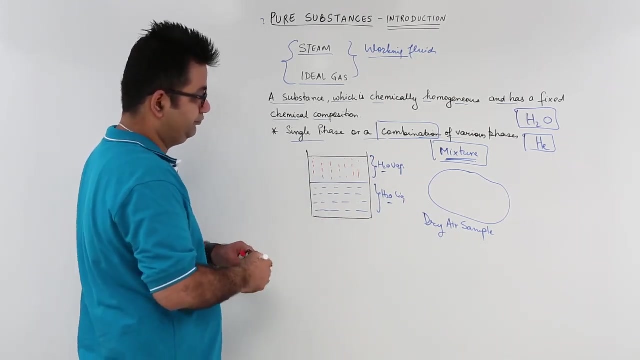 here. So we have a mixture of Water vapour, okay, and this is liquid, liquid water. So a mixture or a combination of water vapour and liquid water there are. it is not a mixture, basically, Okay, so it's a combination of two phases of the same substance, so this entire thing can.